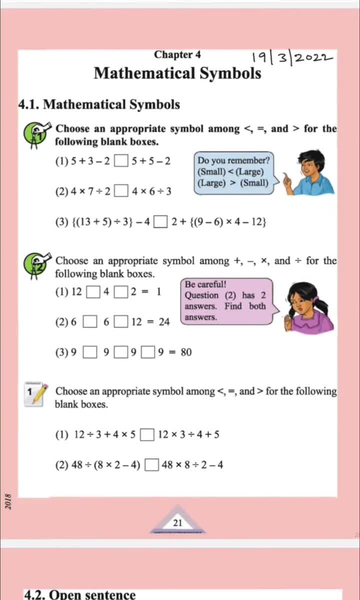 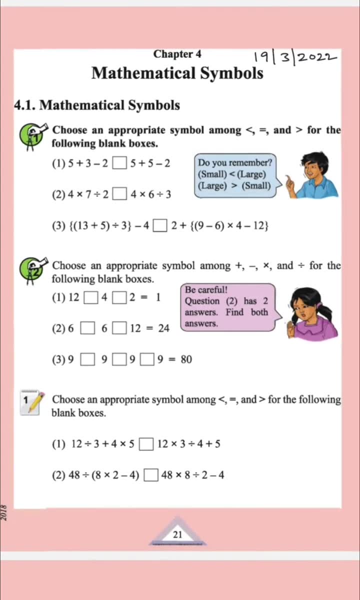 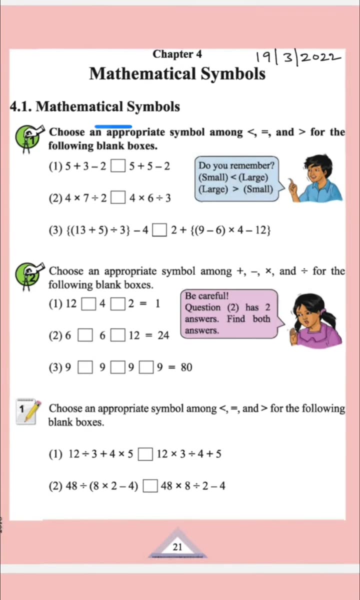 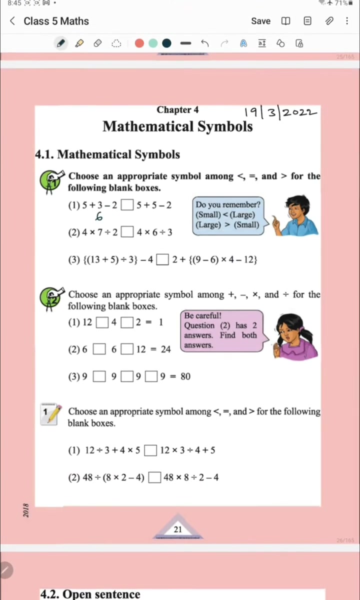 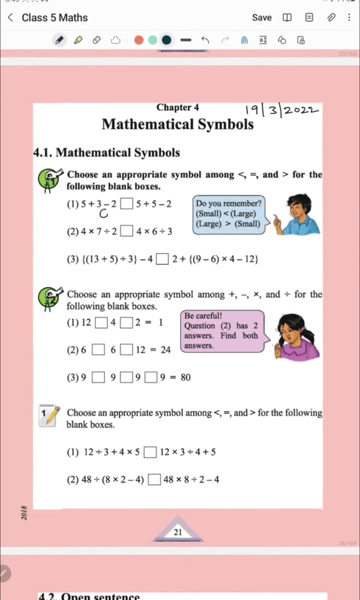 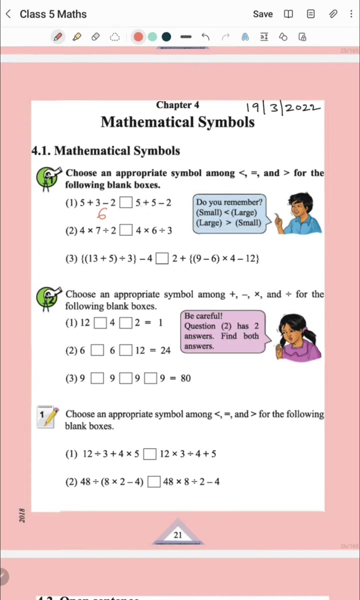 figure out: okay, five plus three minus two, this is what six. we can write it here, i guess: five plus three, eight minus two, six. uh, let's change the color. okay, now this color is fine. fine, this is six. uh, this is eight now, which is greater? uh, six is less. 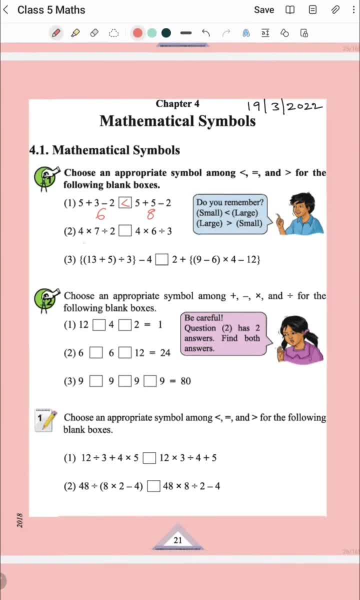 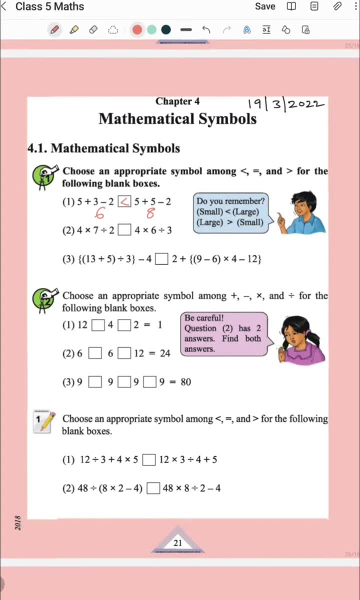 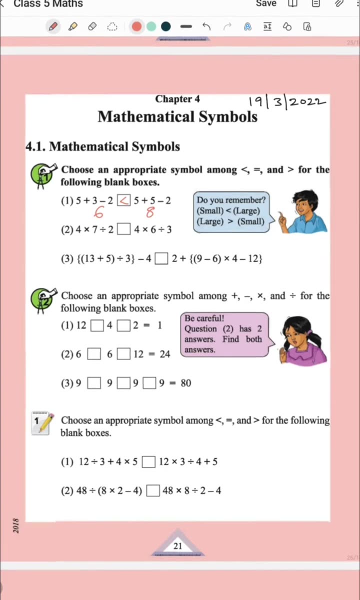 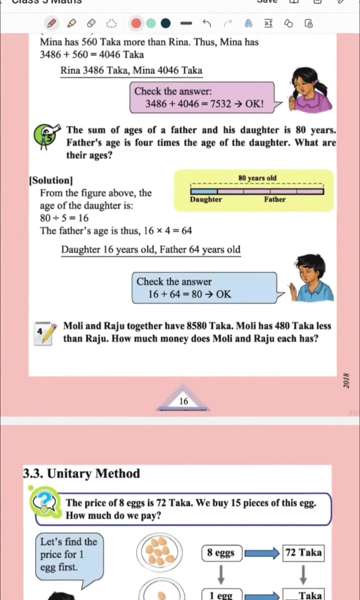 than eight or eight is greater than six. now this one, seven by two, four into seven divided by two, if you remember rightly from the previous lesson. if you want me to, uh, go back to the previous session, we have an order right. in the previous chapter we discussed about the order of the operations, right? 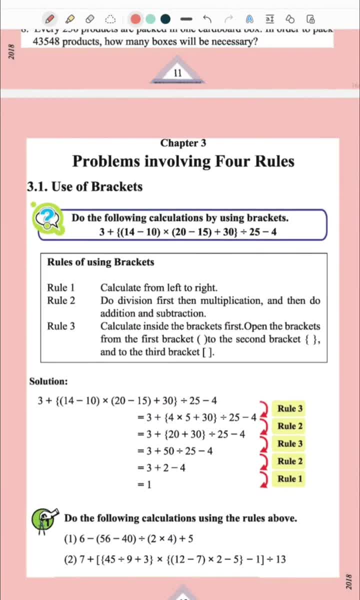 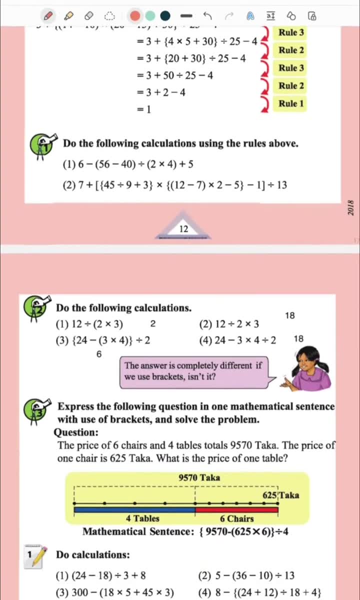 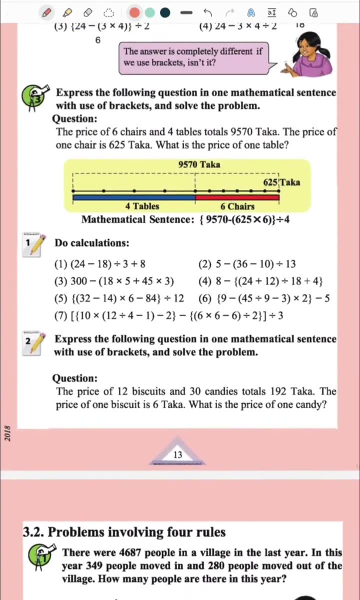 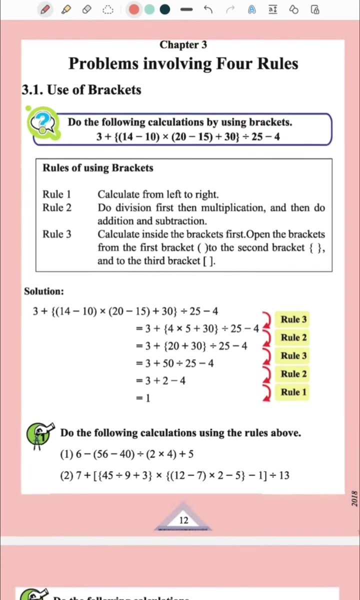 the roots. which one you have to do the first? whichever is there in the black? uh that you have to do first. if there are no brackets, then which one comes first? uh, multiplication or division is less than to correctly, so back to the previous part. that's only change. that's all we're there, okay. so, lastly, we are from x Somer to sería. 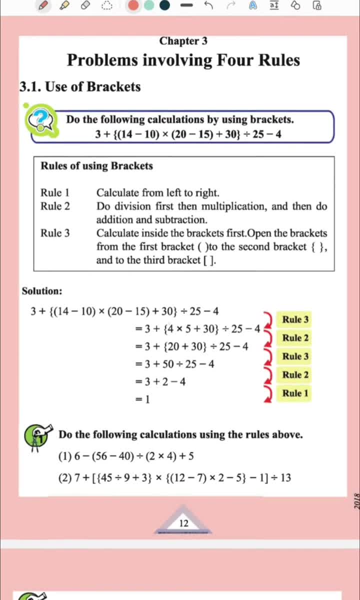 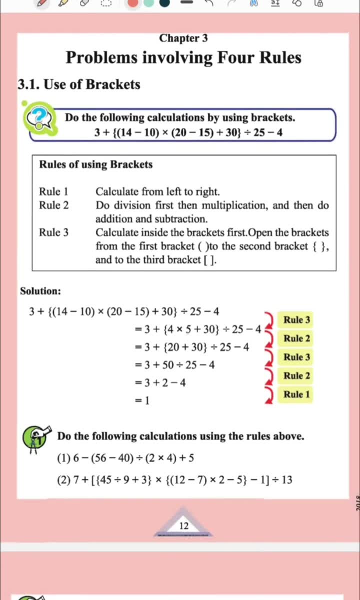 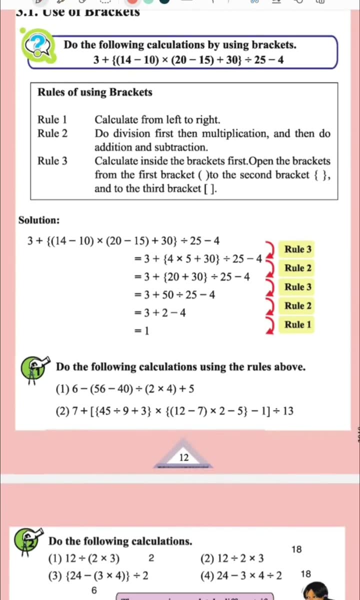 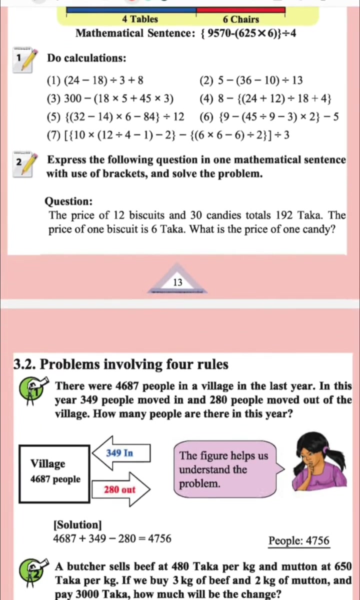 a believing force. x is sorry, very 4 c, lagi thousand n, square root of k. all right, we'll start with the forgetting part. well, yeah, all right, let's have this. okay, comes first. ok, and there is addition and division. you have to do division first. ok, do the division. 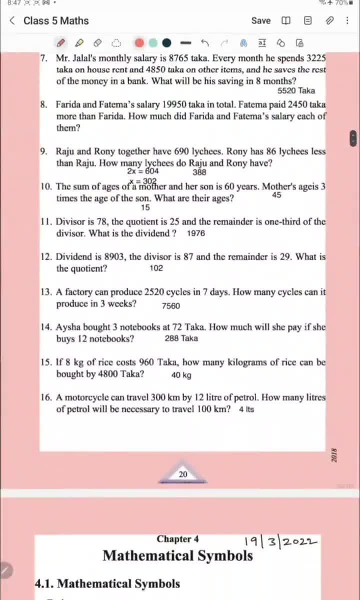 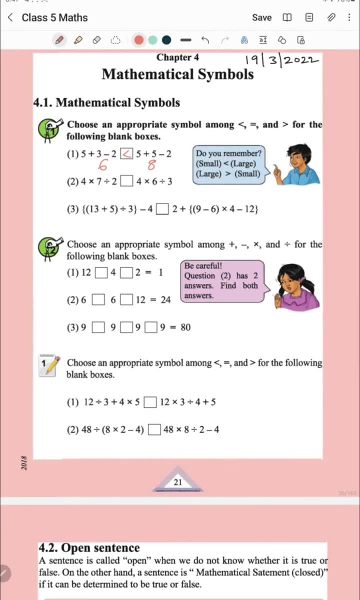 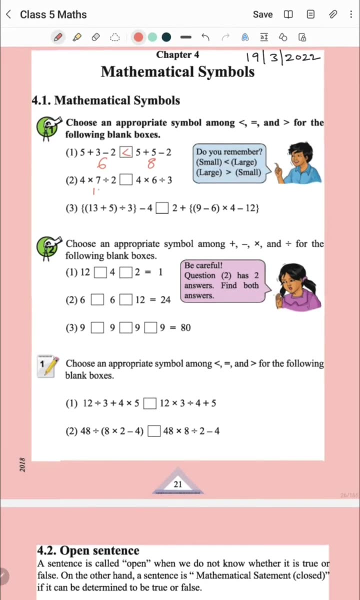 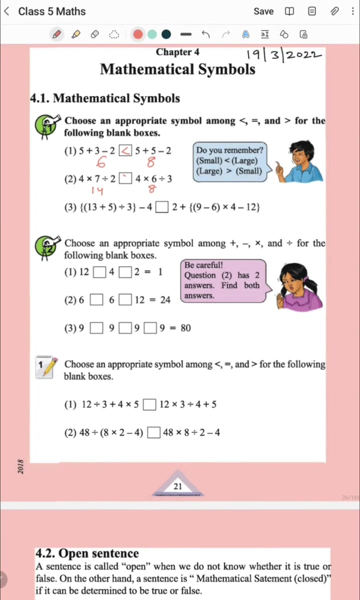 first and then multiplication. ok, that is the rule. then this is: 7 by 2 is 3.5. 3.5 into 4 is how much totalized twenty to fourteen. so this is fourteen, and this is division first. so 2 into 48, which is greater, fourteen is greater than eight. so here bracket is the. 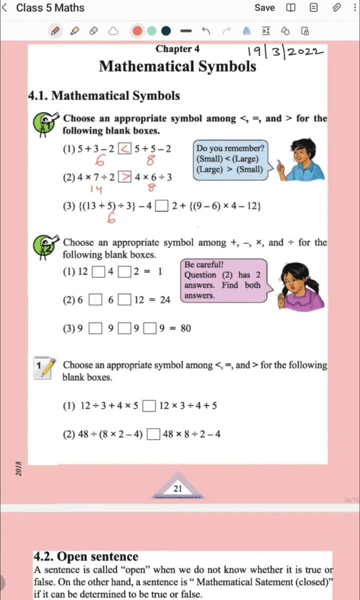 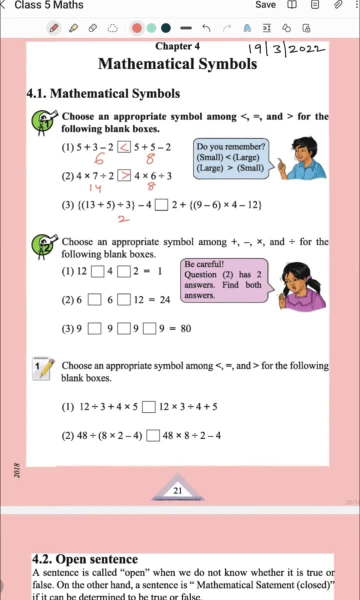 first. so 18 by 3 is 6. here, 6 minus 4 is 2. so this thing will be 2 here and here 9 severe 2.. 17 minus 5 will be 2 here. 9 minus 6 will be 2. 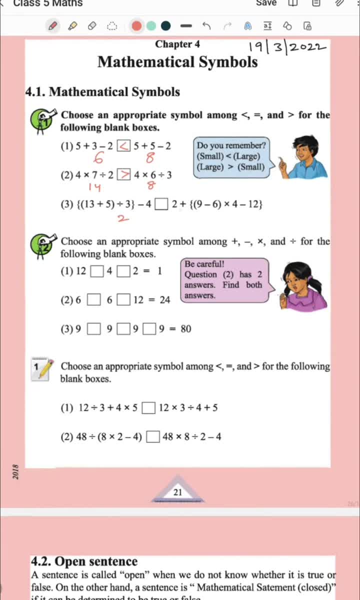 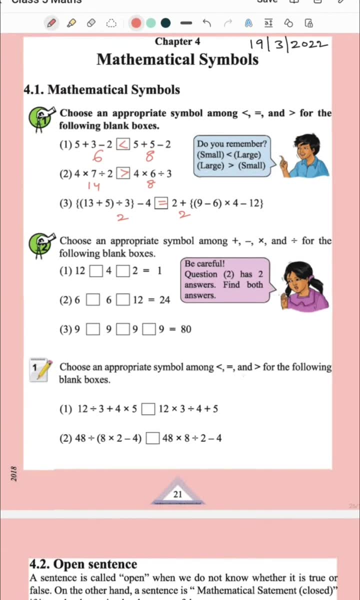 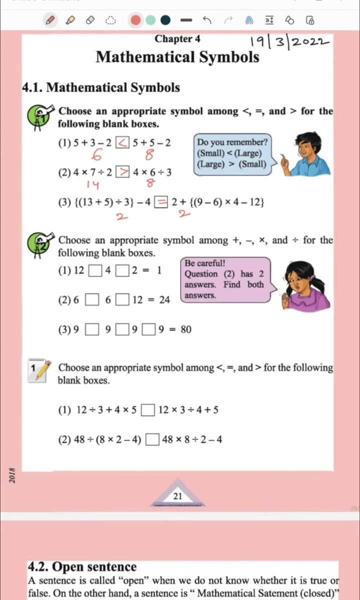 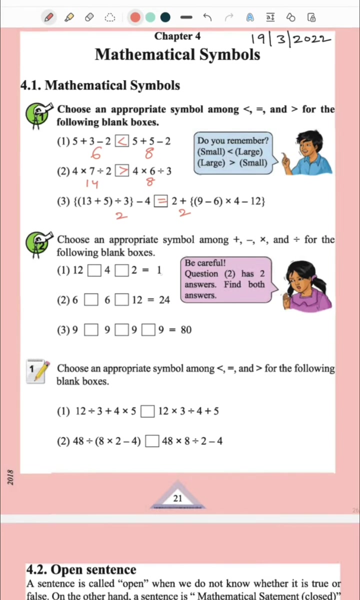 is three. three into four is twelve. twelve minus twelve is zero, so this is two, so both are equal. now the second second one you have to see. okay, she's saying something, be careful. quotient 2 has two answers. find both the answers? okay, we'll see. uh, choose appropriate symbol to get this result, okay. 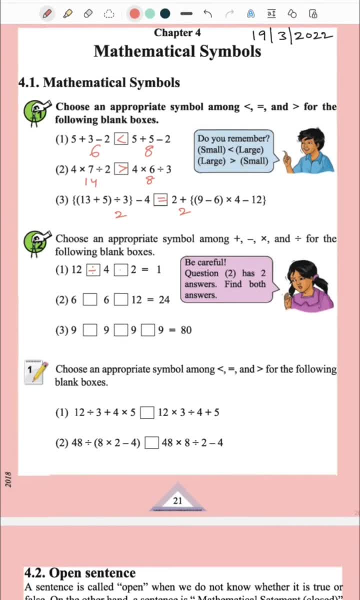 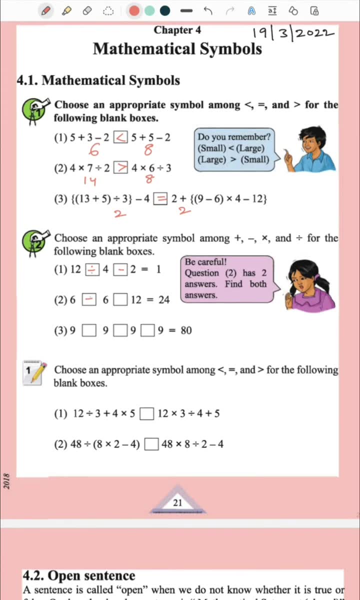 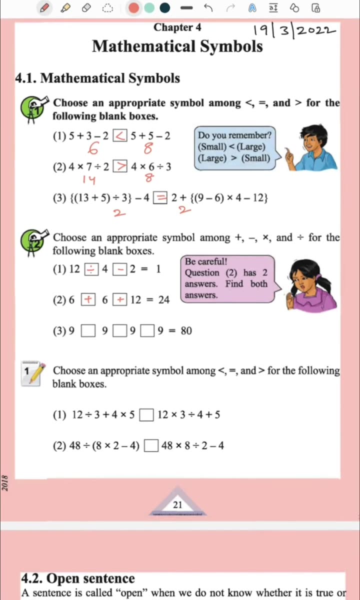 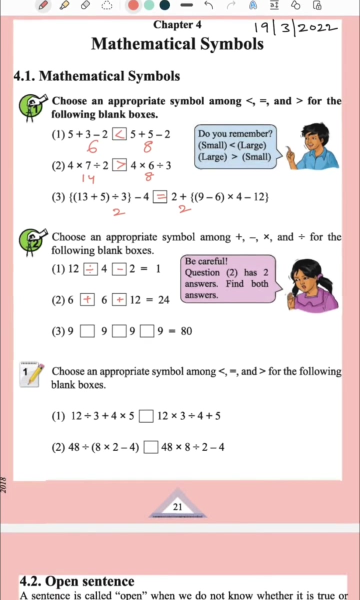 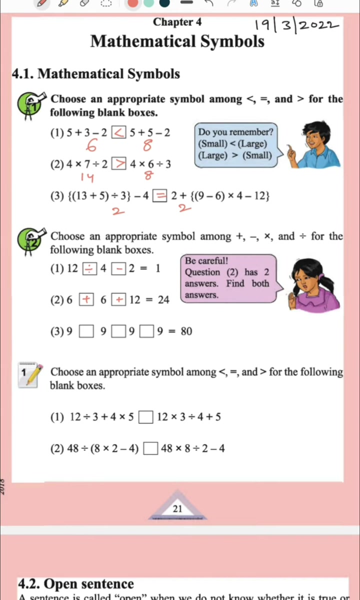 12 by 4 is what? 3, 3 minus 2 is 1. okay, like that: 6 plus 6, uh 12. 6 plus 6, 12, 12 plus 12, 24. that is one answer, i can say. so quotient 2 has both answers, two answers. we need to find both the answers right. 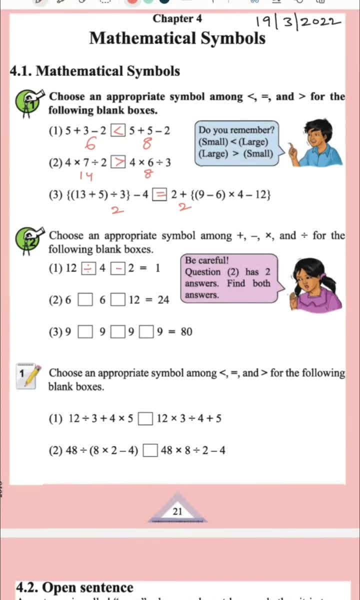 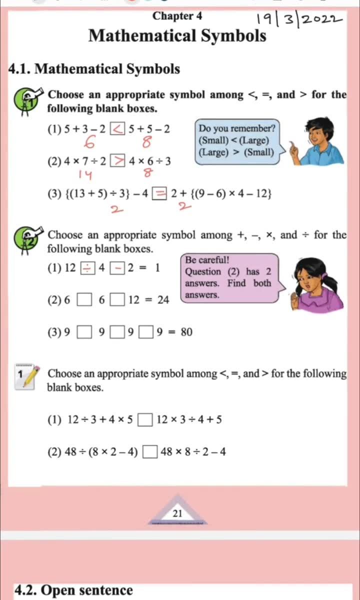 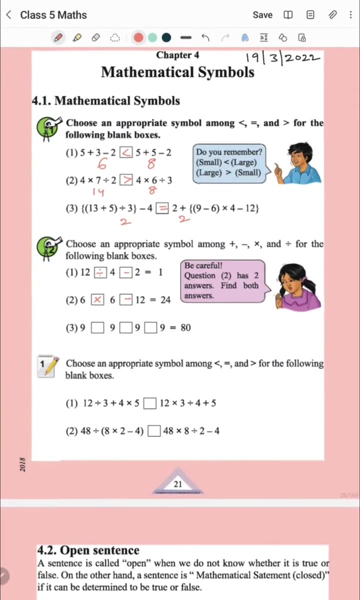 okay, s plus is one answer, because 6 plus 6 is 12, 12 plus 12 is 24.. right now, you need to find the other answer as well, right, okay? 6 into 6 is 36, 36 minus 12 is 24, right? this could be the another question. 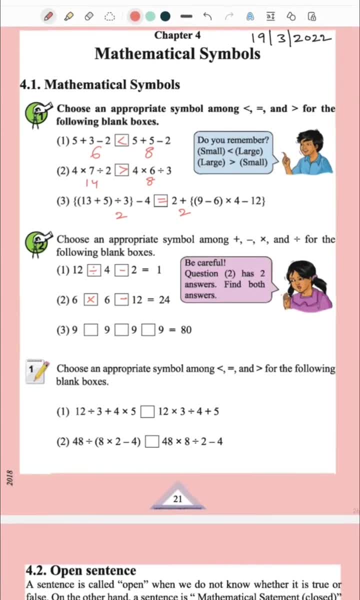 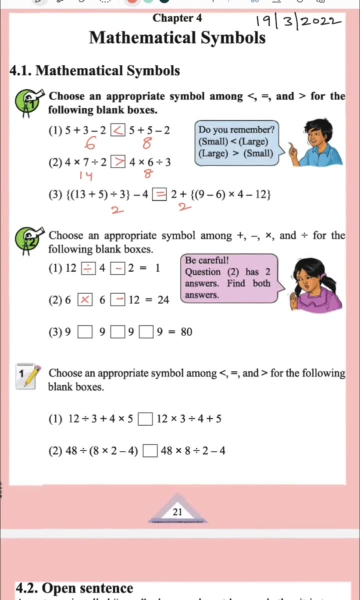 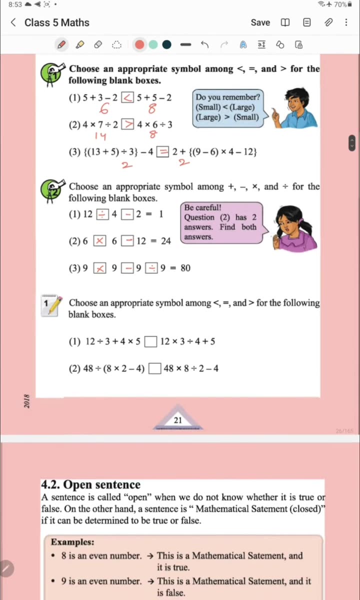 right, this could be the another question. right, this could be the another question. um, here you can see. 80 is there in the right hand side. how to get 80 from all nines? okay, 9 by 9 is 1, 9 into 9, 81, 81 minus 1 is 80.. okay, choose appropriate symbol less than equal to. 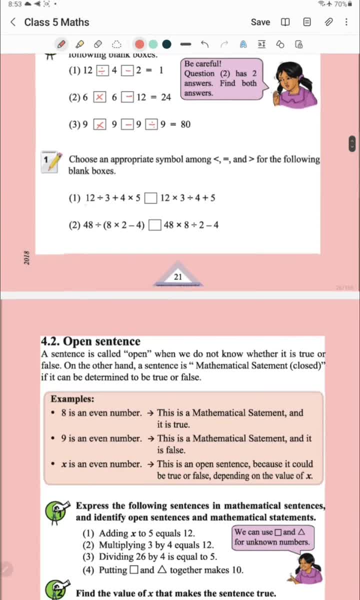 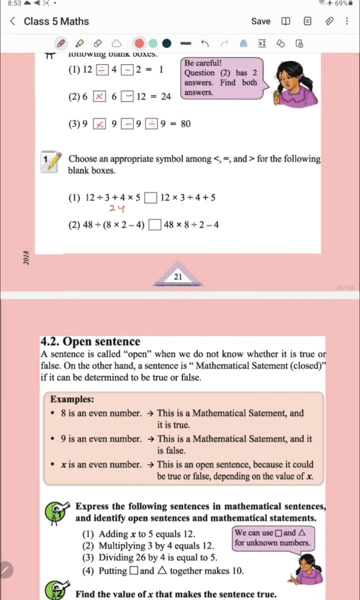 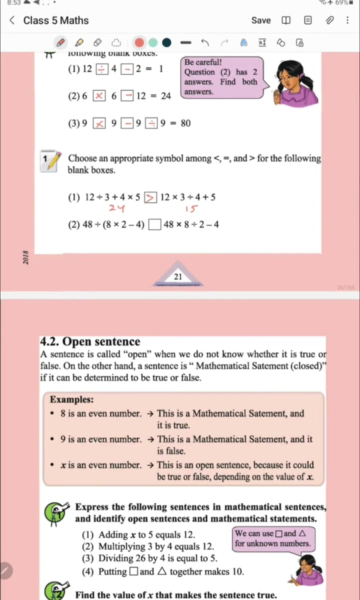 greater than now falling boxes: 12 by 3, 4, 4 into by 20, this is 24.. that is 9 plus 5, 14. so this is greater than 8 is 16 minus 4, 4. 48 by 1 is 4. this is 8 by 2 and 48 into 4.. 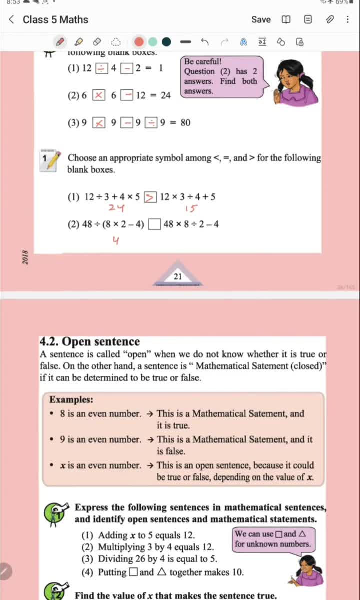 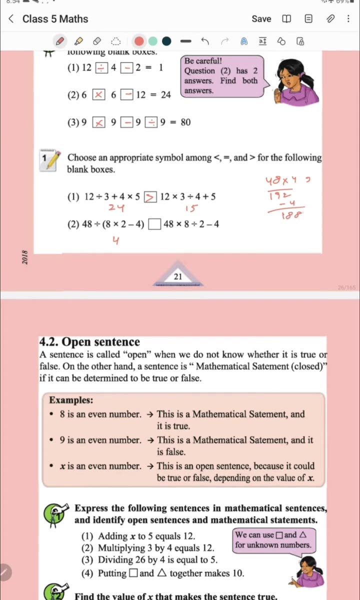 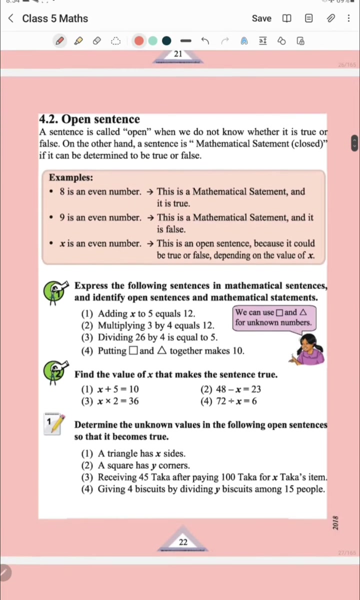 this is 8 by 2, 4 and 48 into 4.. 48 into 4 is 4,, 8 is 32,, 3 is 4,. 16 plus 3 is 19,. 192,. 192 minus 4 is how much 188, so this is 188,. so this is rather than the open sentence. a sentence is called open when we do not know whether it is true or false. 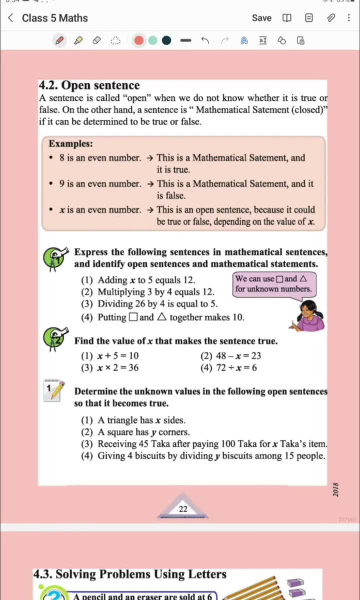 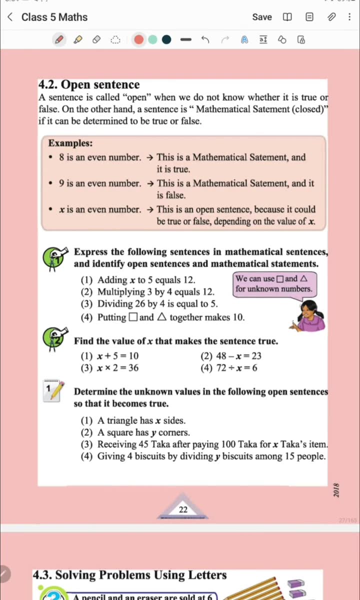 on the other hand, a sentence is a mathematical statement closed if it can be determined to be true or false. 8 is even number. this mathematical statement is true. 9 is even number. this is false. x is even number. this is open sentence because it could be true or false depending upon the value of x. 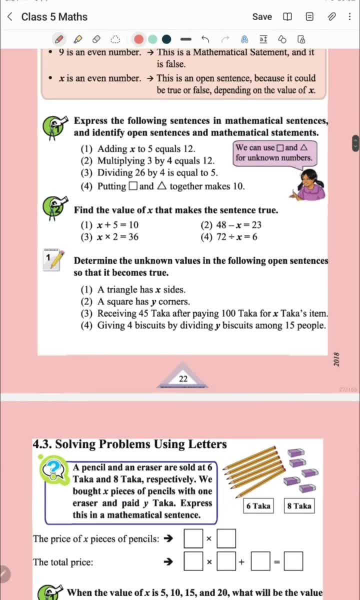 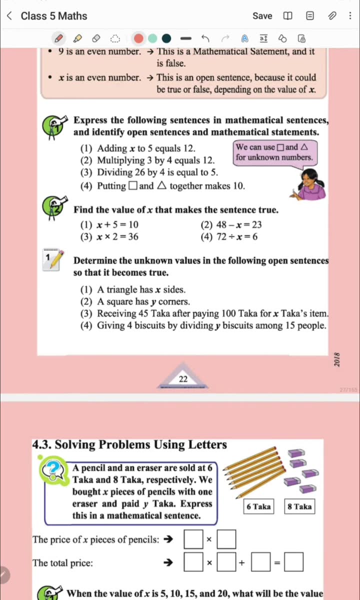 so express the following sentence in mathematical sentences and identify the open sentences and mathematical statement. we can use a straight line and for unknown number: okay, adding x to 5 equals 12,. multiplying 3 by 4 equals 12, dividing 26 by 4 is equal to 5, this is false, clearly false. this is true. 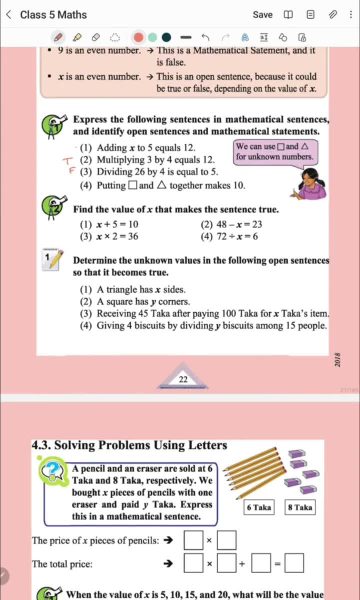 now, this is open statement. first one is: this is open statement: putting this and this together makes 10, that is also a open statement. find the value of x. that makes the sentence true. okay, here you can see: x plus 5 is 10. 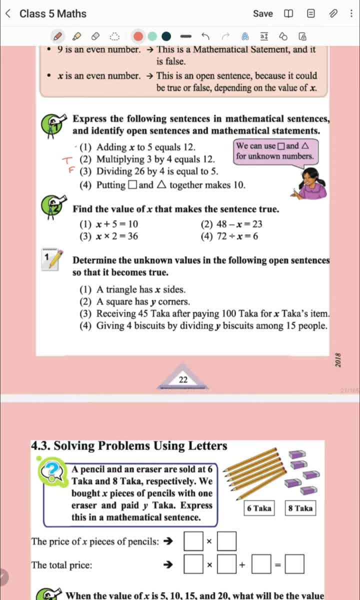 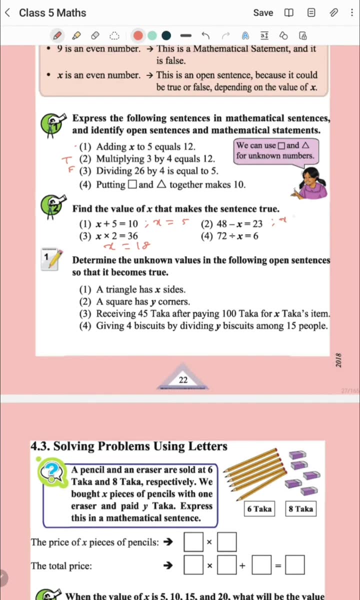 so x is what. x is 10 minus 5, that is 5. here x into 2 is 36. so x equal to 36 by 2, that is 18. and here x equal to 48 minus 23. how much 48 minus 23: 15? 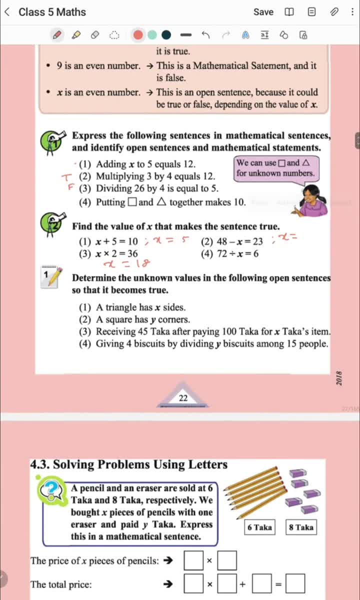 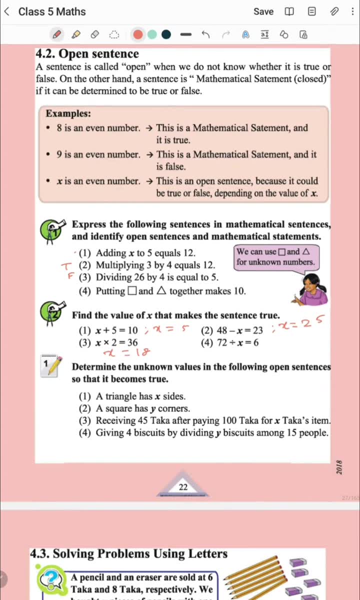 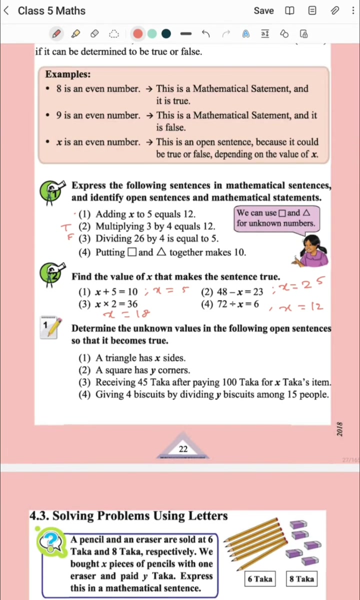 15 or 25, 25, so that would be 25. okay, 72 by x is 6. so x equal to 72 by 6, that is 12. okay, determine the unknown values of the following of the following: x is equal to 32 by 6, that is 12. 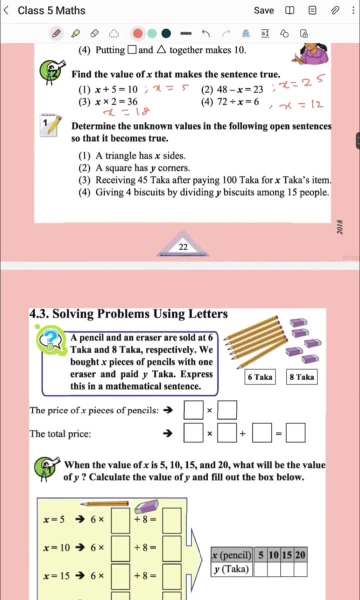 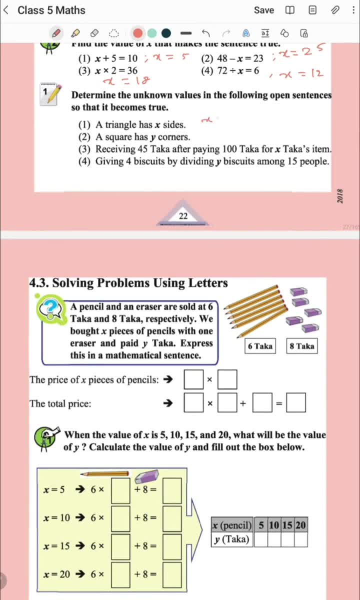 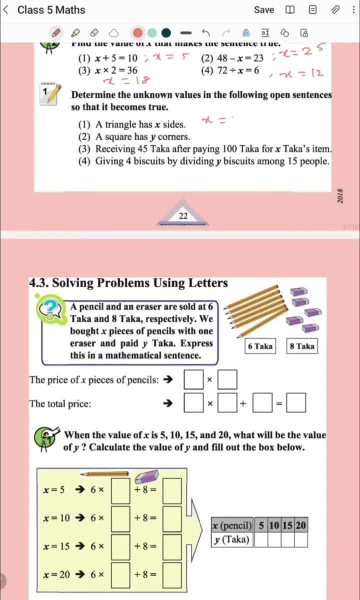 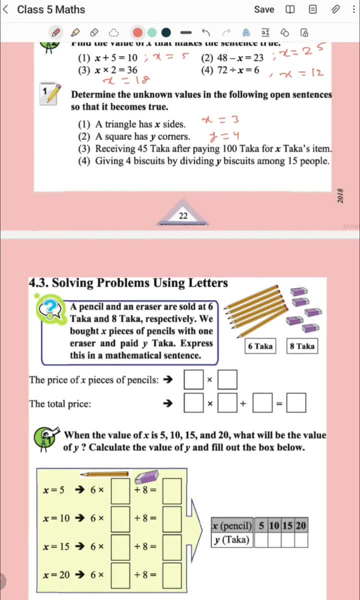 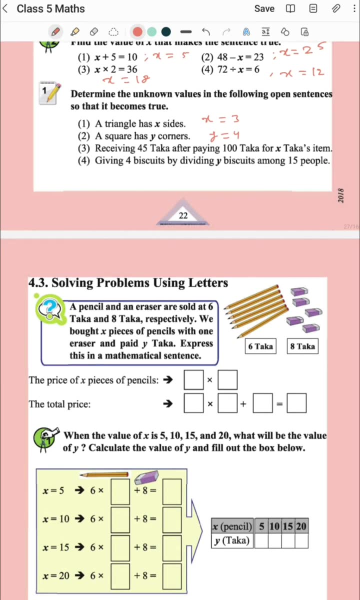 okay, determine the unknown values of the following: x is equal to 32 by 6, that is 12. okay, determine the unknown values of the following: x is equal to 32 by 6, that is 12. okay, determine the unknown values of the following: So what is xthaka here? 100 minus 45, that is 55, that is 55thaka. giving 4 biscuits by: 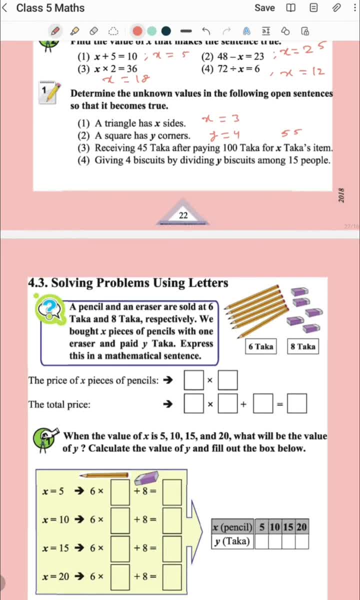 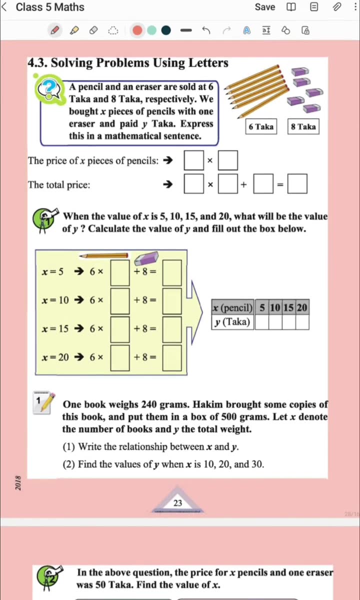 dividing y biscuits among 15 biscuits, so y is how much 15 into 4, 60, solving problem using letters. so pencil and arranger have sold at 6thaka and 8thaka respectively. we bought x pieces of pencil with one arranger and paid ythaka. express this in a mathematical sense. 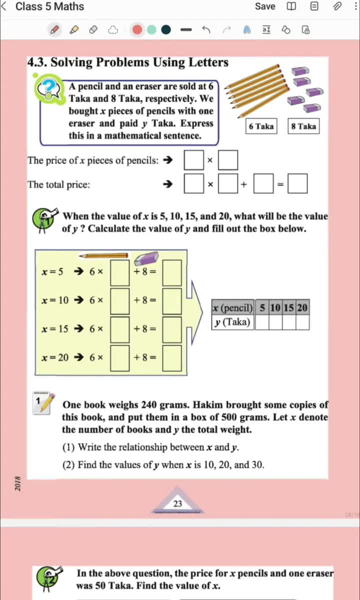 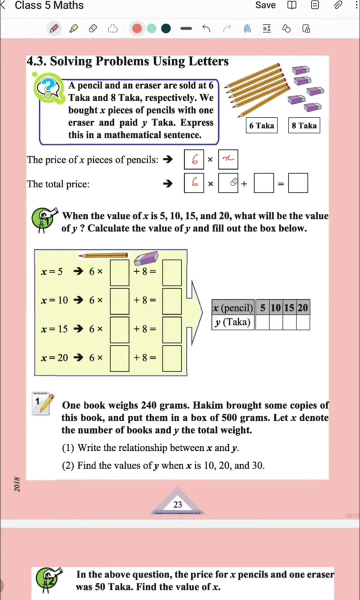 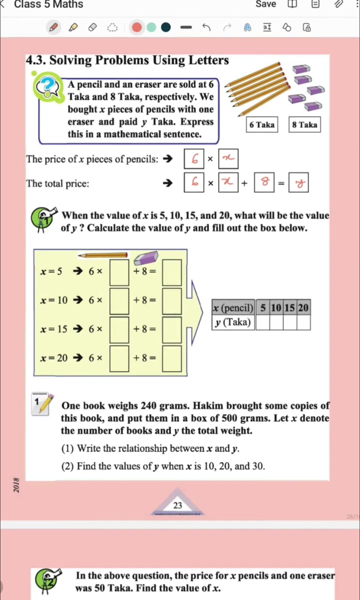 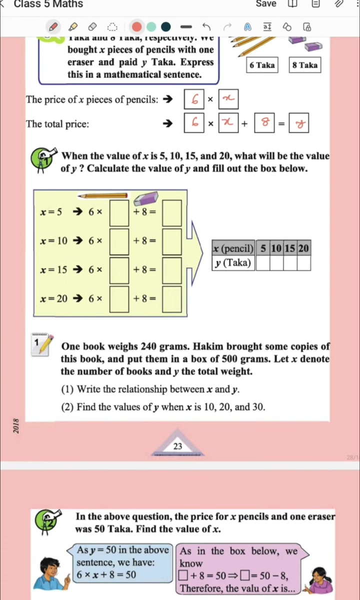 the price of x pieces of pencil. so all pencil is 6thaka. so all pencil is 6thaka. so 6thaka next is dotestaste, dotestaste. this way, 6thaka, this way. when the value of x is 5, 10, 15, 20, what will be the value of y? calculate the value of y. 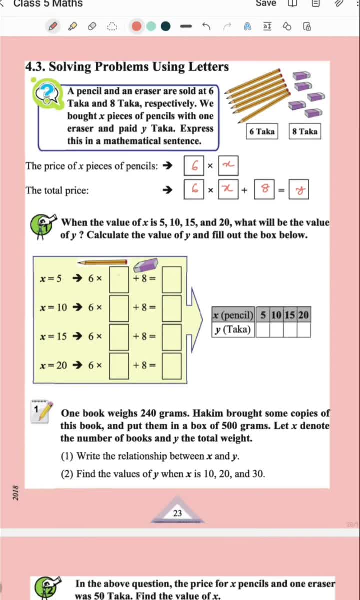 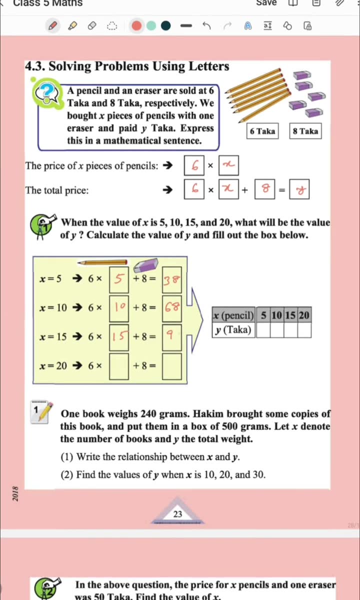 fill out the box below: x 5 y is 30 plus 8, uh, 38. x 10 y is 60 plus 8. 68 x 15 y is 90 plus 8, 98 and this is 20- 128. okay that you can fill it out here okay. 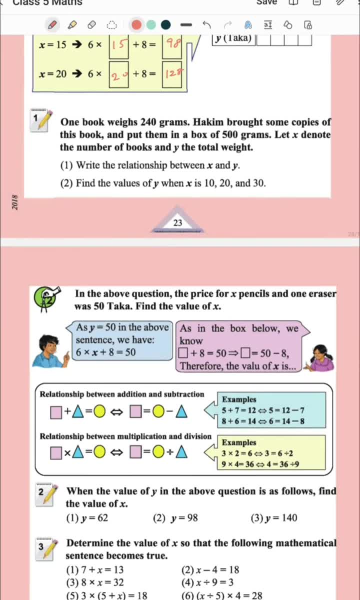 one book base is 240 grams. hakim bought some copies of this book and put them in a box of 500 grams. let x denote the number of books and y is the total weight. write the relation between x and y. one one book weighs 240 grams. 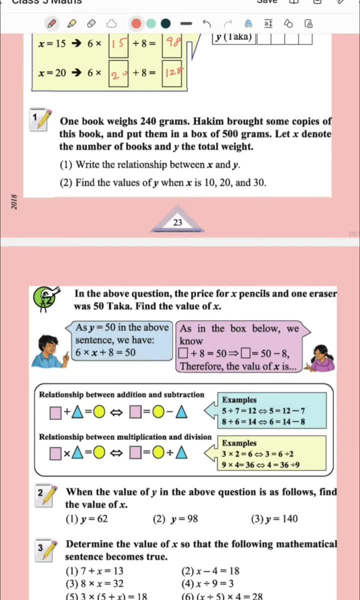 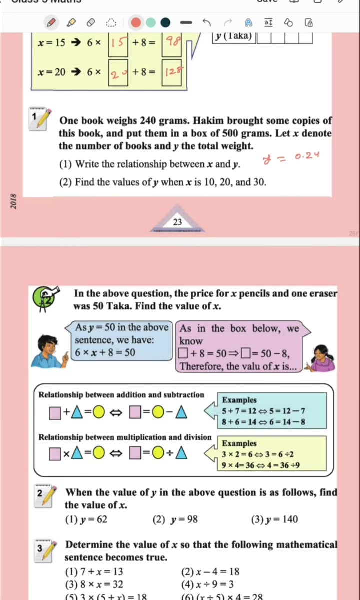 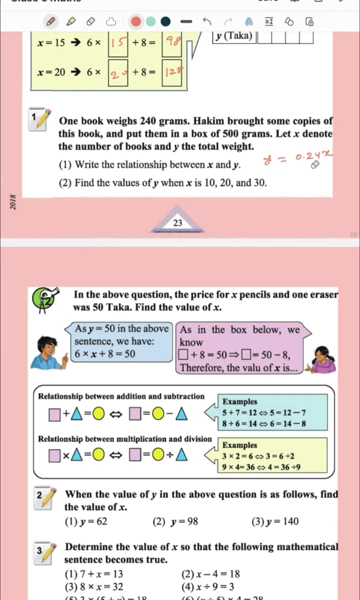 put them in the box of 500 grams. let x denote the number of books and y is the total weight. got to think: find 240, 240, okay, okay, so okay, friends say in the above question, the price of x pencils and one eye razor was 50 thakar, find the value. 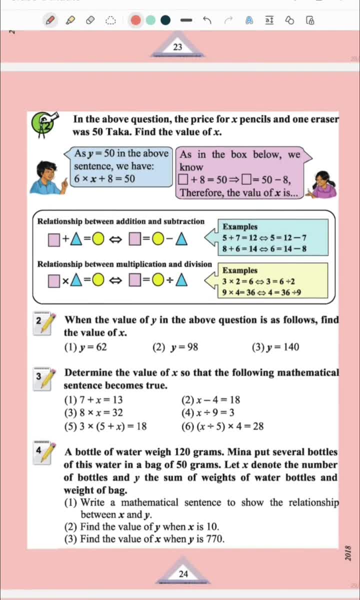 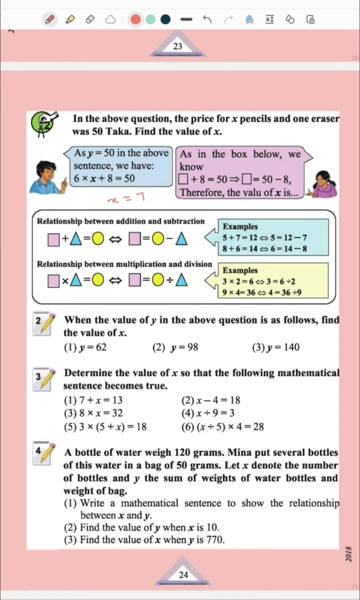 of x, that is 6x plus 8, is 50. then 6x is 50 minus 8, that is 42. 42 by 6. how much 7? so x value is 7, okay. so 5 plus 7 is 12. 12 minus 7 is 5. 8 plus 6 is 14. 6 minus 14 is 14 minus 8 is 6, okay. 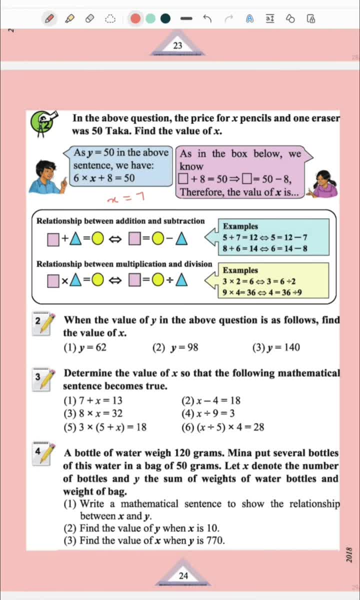 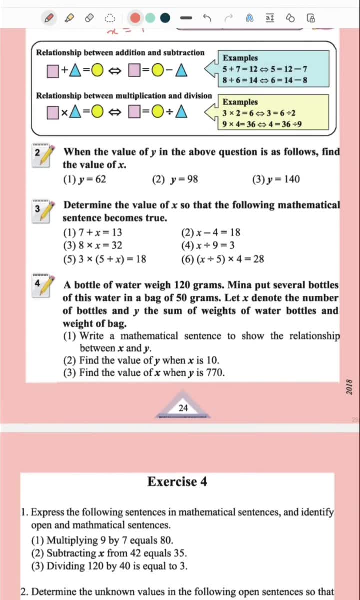 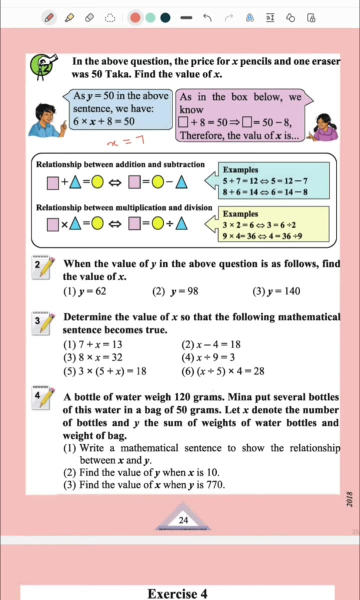 that is division. now, urgent statement can also be written as subtraction statement. okay, when? the value of what? when? the value of y in the above question is as follows: find the value of x, y equal to 62. find x- you can put it here- and find out the value of x. okay, determine the value of x. 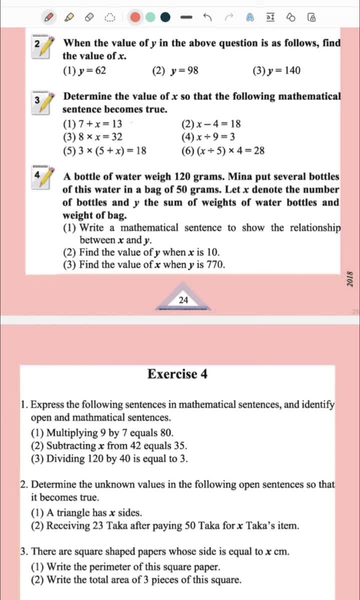 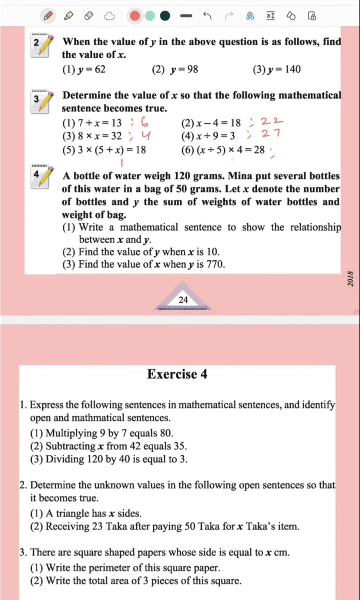 so that the following mathematical sentence becomes true: here x equal to 6 and here it is 4. here the equation is written: here and here it is 6 plus 3, Nation. so now, if y is equal to 3, achi8 plus誰 harder than, luckily, seine 6? we have 123 by 3 is 18 minus 4, sorry. 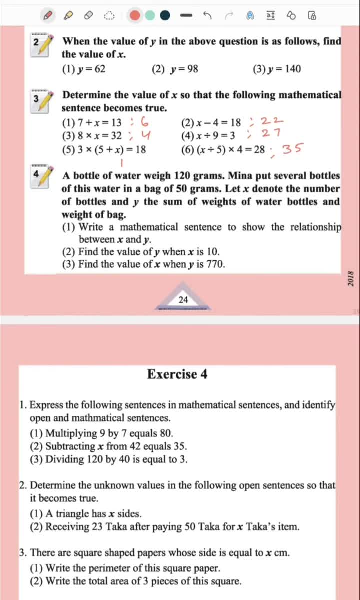 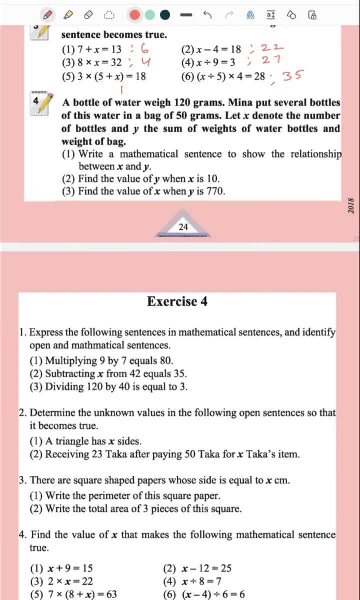 19 plus 4, 22. here it is 3 into 9, 27. here it is 127, 35, so here it is 35. 35 bag of 50 grams. Let x denote the number of bottles and y is the sum of weights of water. 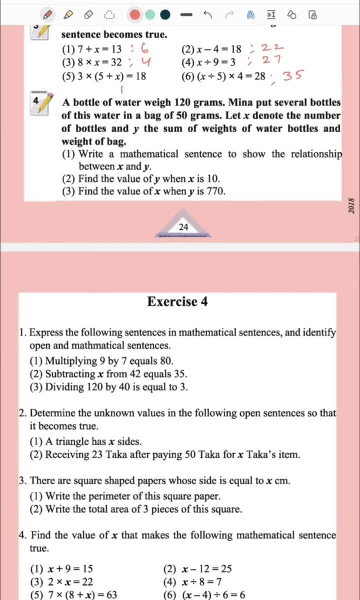 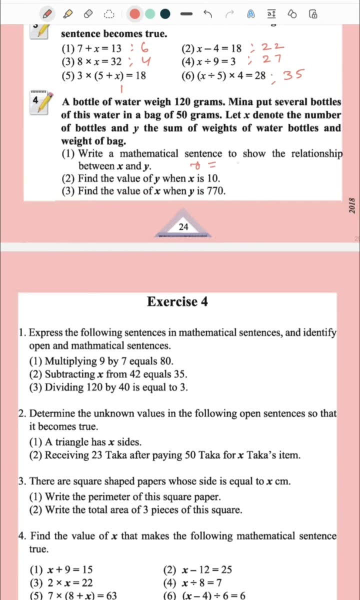 bottles and weight of the bag. Write the mathematical sentence showing the relationship between x and y: y equal to 120x plus 50.. Find the value of y when x is 10.. When x is 10, this is over etol 50, etol 50.. Find the value of x when y is 770.. When y is 770, 770 minus. 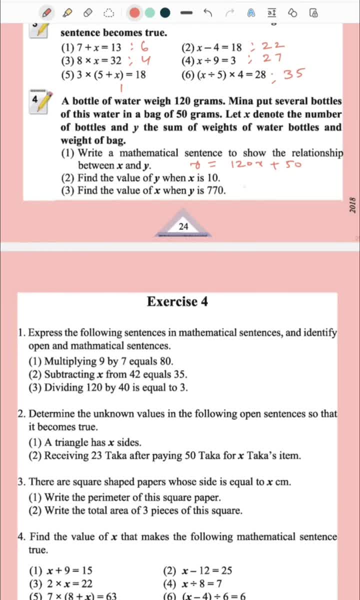 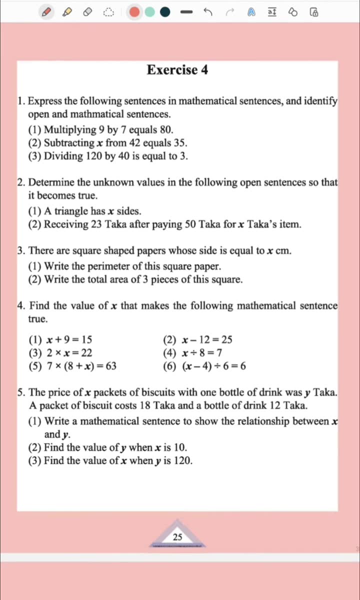 50,, that is 720.. Yes, 720.. x equal to 720 by 120. 6.. Okay, Right, We came to exercise 4.. Let's see the exercise 4.. Express the following sentence in mathematical sentences and identify open and mathematical sentences Multiplying: 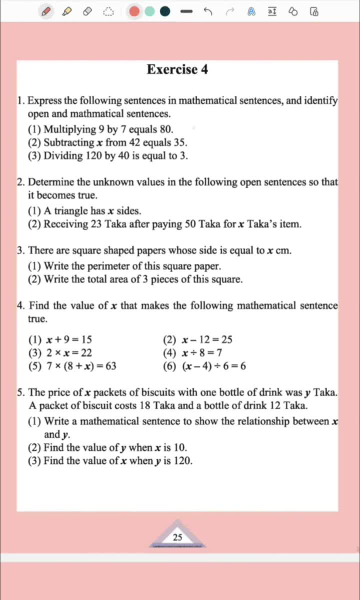 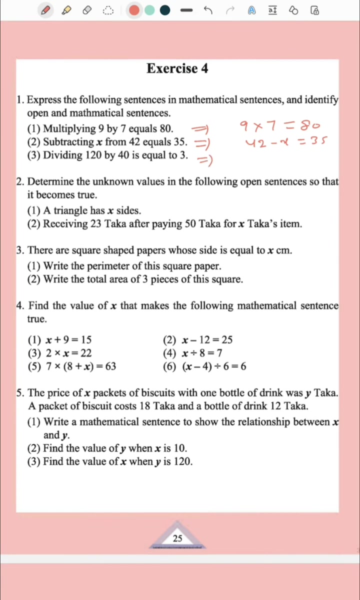 9 by 7 equals 80.. Multiplying 9 by 7 equals 80.. This is not true. Okay, Subtracting x from 42.. 42 minus x equal to 35.. This is a mathematical statement. Okay. Dividing 120 by 40 equal. 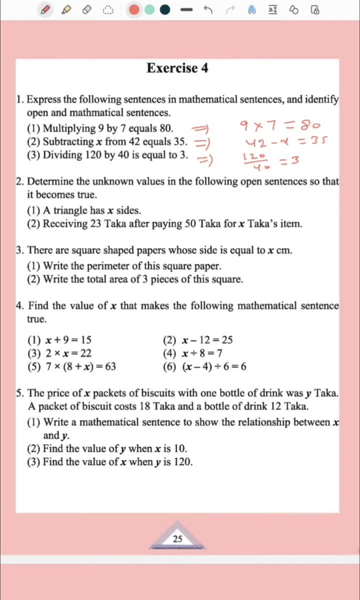 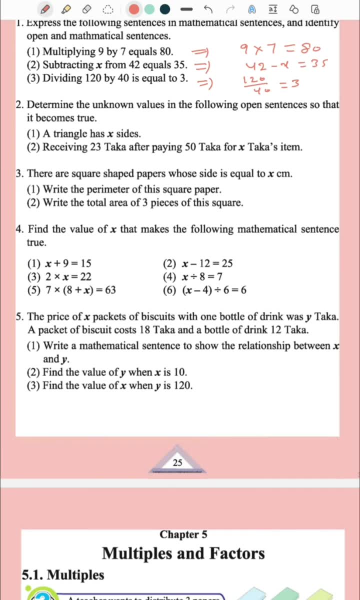 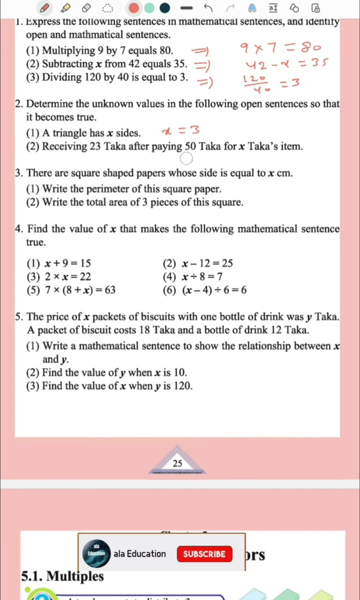 to 3.. This is also a mathematical statement. because this is true, Determine unknown value of the following open sentences so that it becomes true: The triangle has x sides When x is 3, this is true, wny. What is x then? 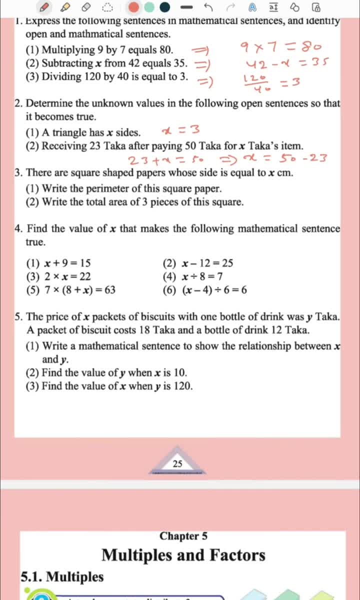 20 minusles Lazier When you place an object in the labour force on a surface. assuming 50 holiday guys for x others, pressure item. Now what is the value of x then receiving 23,, 50 minus23.. 23 plus x equal to 50. Okay, So what is x then? 23,, 50,, 23.. 50 minus 23, what is? 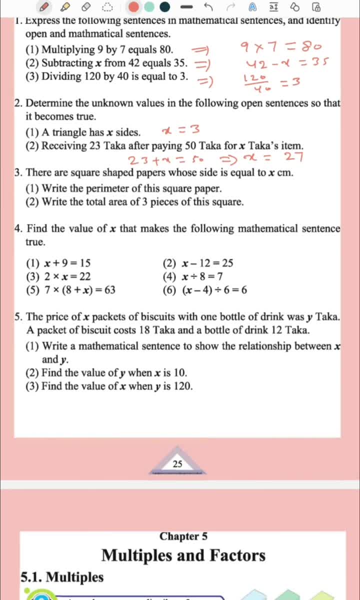 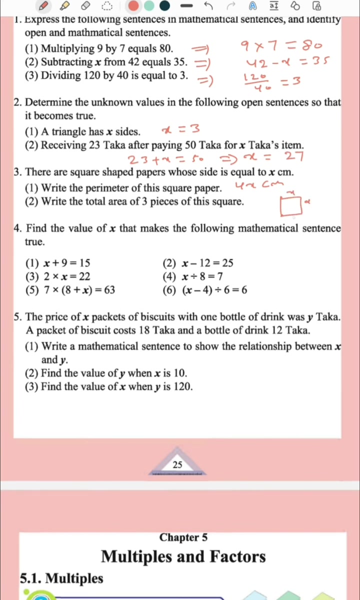 27, right, so this is 27, tata. there are square shaped papers whose side is equal to x cm. write the perimeter of this square paper 4x 4x cm, because square has four sides and all four sides are equal. okay, x plus x plus x plus x. like this, this is a square: x x, x, x when you start from. 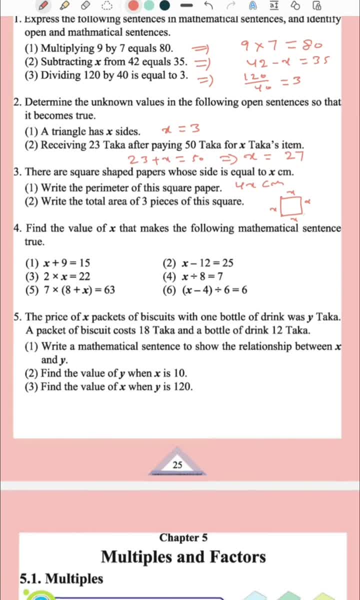 here or run run along this line: x in x cm. x cm, 2 x cm plus x, 3 x cm plus x 4 x cm. you started here and you ended here. that is the perimeter will be nothing but 4x. write the total area of three. 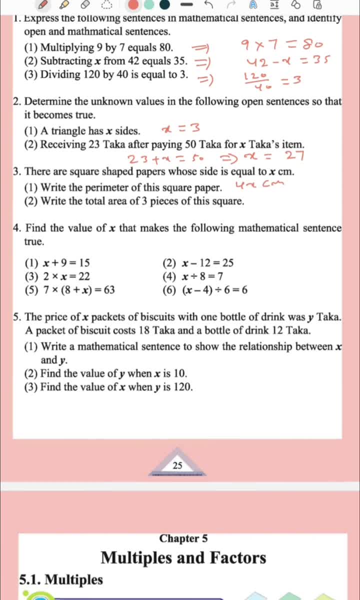 pieces of the square. total area of three pieces of this square one piece area is x square. three pieces is three times x square. x square plus x square plus x square is nothing but 3 times x square cm square in the centimeter square square centimeters find. 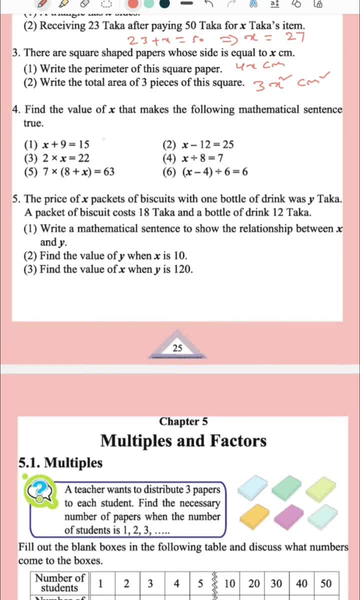 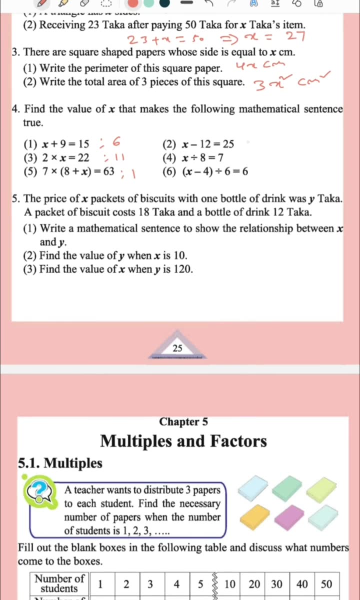 the value of x. that makes the following mathematical sentence true: okay, fine, x quize should be 6 here year. it should believe in your 9 minus 8, 1. okay, 8 plus 1, 9, 9, 9, 7, the 53 here, it is 37 here. 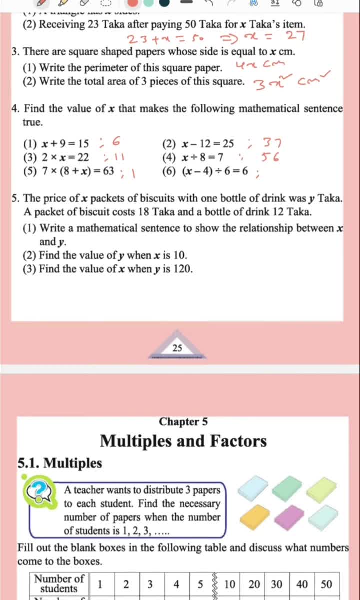 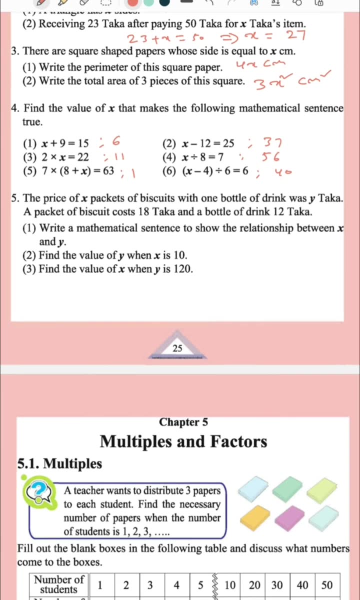 it is 7 into 8, 56.. 36 plus 4, 40.. 40 minus 4, 36.. 36 plus 6 is 6.. The price of X packets of biscuits with one bottle of drink was Y taka. The packet of biscuits cost 18 taka. 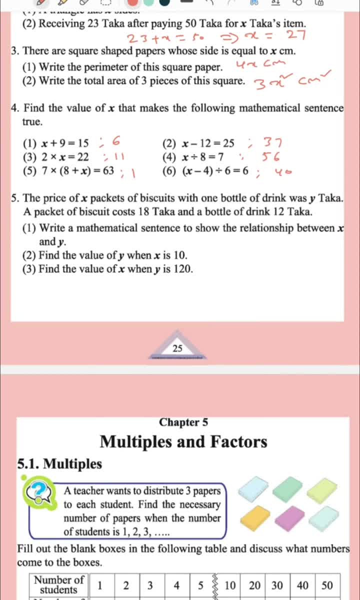 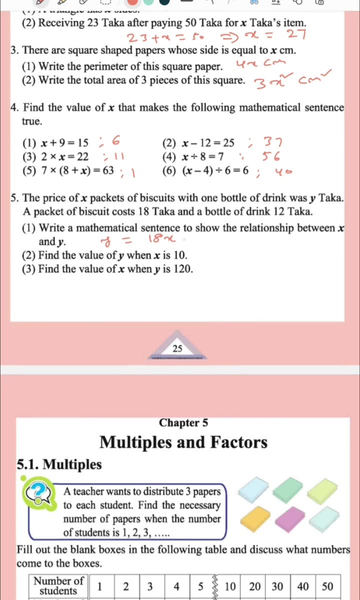 and a bottle of drink 12 taka. Write a mathematical sentence to show a relationship between Y and X. Y is the total price. X packets of biscuits: 18 each. So 18 into X packets with one bottle of drink. One bottle of drink is 12 taka, So 18X plus 12 is the relation. 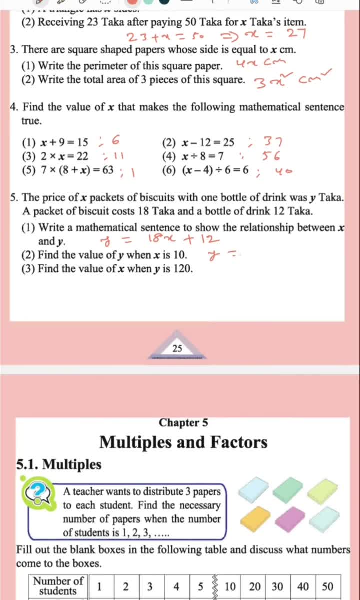 Find the value of Y when X is 10.. When X is 10, Y equal to 18 into 10 plus 12, 192 taka That you have to write Taka. also you have to write: Find the value of X when Y is 1. 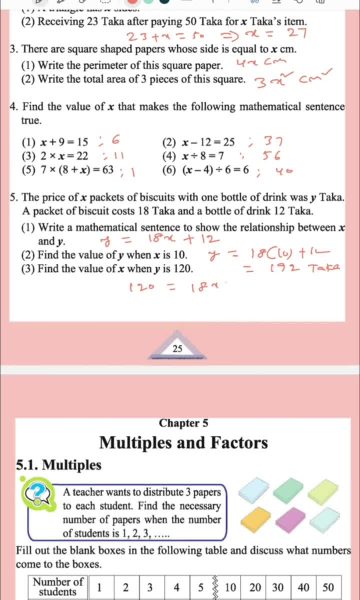 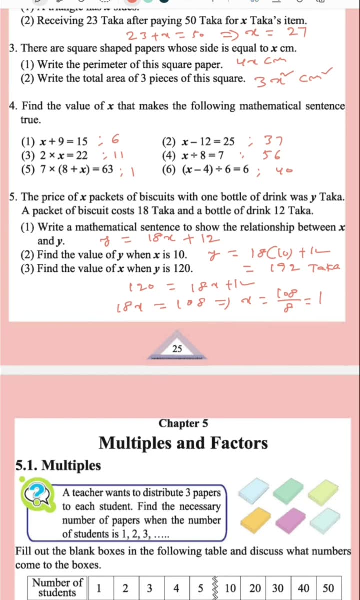 to 2.. 120. Okay, 120 equal to 18X plus 12.. So 18X equal to 120, 1, 10, 108.. So X equal to 108 by 8.. 8 x 1 is 8.. 8 x 6 is 48.. No, that is not correct. 8 x 1 is 8..